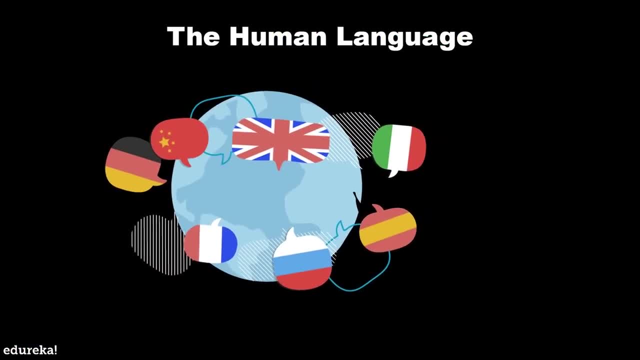 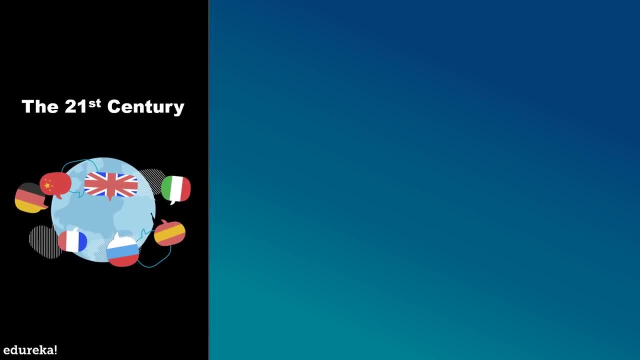 the human language. it is one of the most diverse and complex part of us, considering a total of 6,500 languages that exist, So coming to the 21st century. according to the industry estimates, only 21% of the available data is present in the structured form Data. 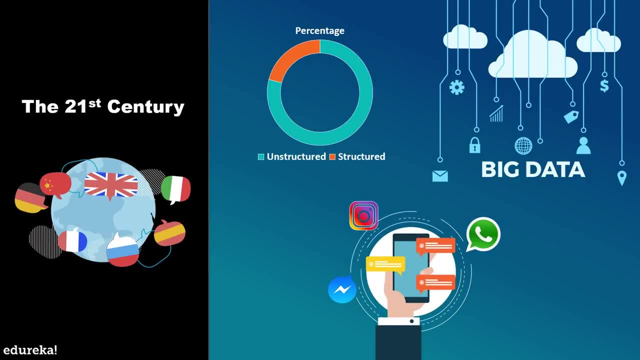 is being generated as we speak, tweet and send messages on WhatsApp or the various other groups of Facebook, And majority of this data exists in the textual form, which is highly unstructured in nature. Now, in order to produce significant and actionable insights from this data, it is important to get acquainted with the techniques. 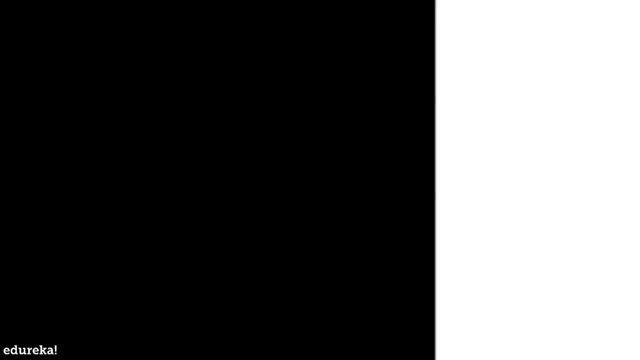 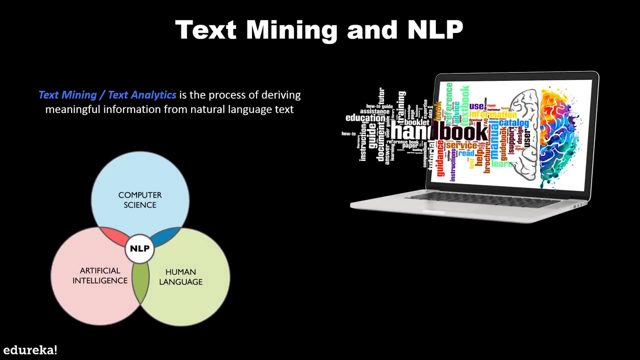 of text analysis and natural language processing. So let's understand what is text mining and natural language processing? So text mining or text analytics is the process of deriving meaningful information from natural language text. It usually involves the process of structuring the input text, deriving patterns within the structured data and finally, evaluating and. 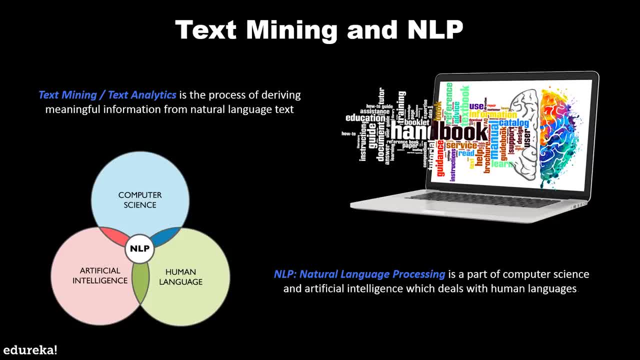 interpreting the output. Now, on the other hand, natural language processing refers to the artificial intelligence method of communicating with an intelligent system using the natural language. As text mining refers to the process of deriving high quality information from the text. the overall goal is here to essentially turn the text into data analysis via the application. 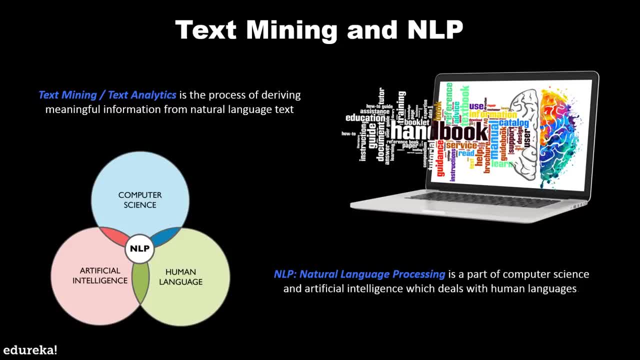 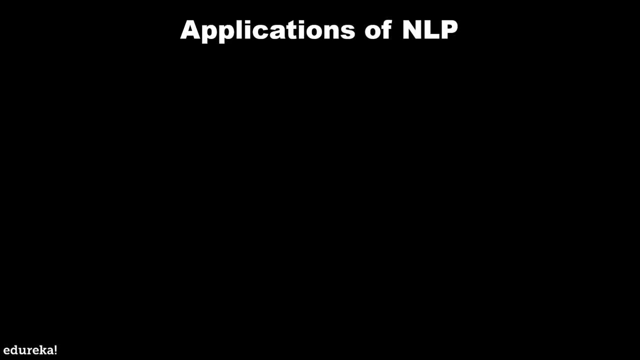 of natural language processing. That is why text mining and NLP go hand in hand. So let's understand some of the applications of text mining or natural language processing. So one of the first and the most important applications of natural language processing is sentimental analysis, Be it Twitter sentimental analysis or the Facebook sentimental analysis. 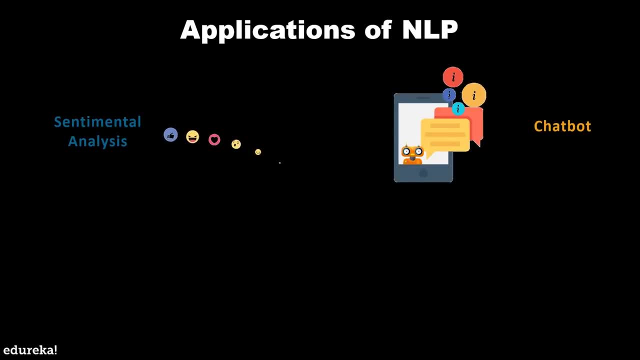 it's being used heavily Now. next, we have the implementation of chatbot. Now you might have used the customer chat services provided by various companies, and the process behind all of that is because of the NLP. Now we have speech recognition, and here we are also. 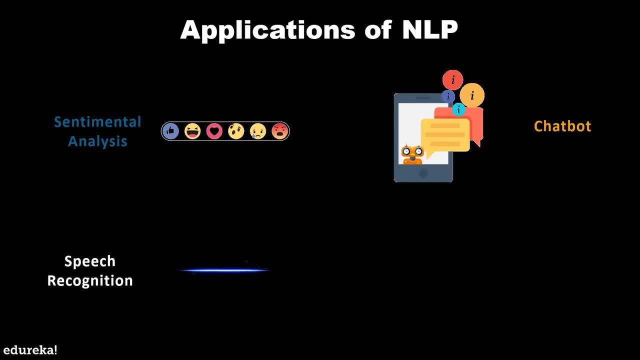 talking about the voice assistants like Siri, Google Assistant and Cortana, and the process behind all of this is because of the natural language processing. Now, machine translation is also another use case of natural language processing, and the most common example for it is the Google Translate, which uses NLP to translate data from one language to another. 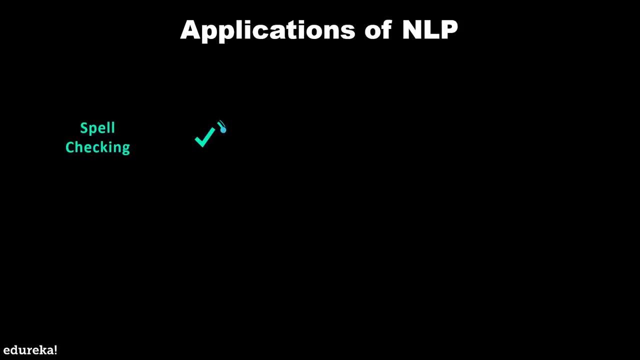 and that, too, in the real time Now. other applications of NLP include spell checking, keyword search and also extracting information from any doc or any website. And finally, one of the coolest application of natural language processing is advertisement matching, Basically recommendation of ads based on your history. 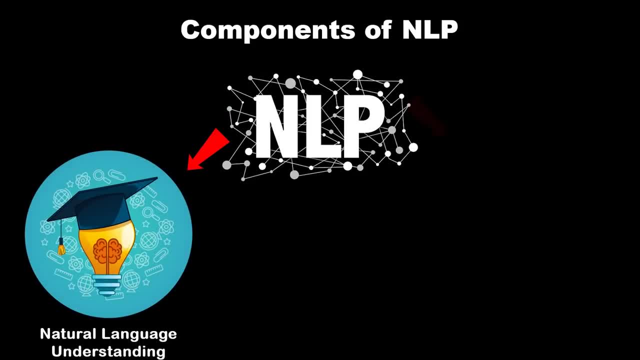 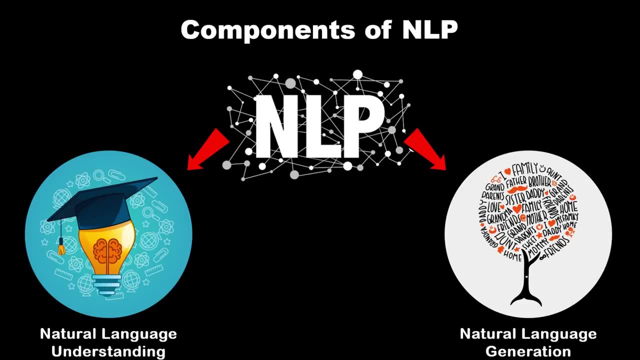 Now NLP is divided into two major components, That is, the natural language understanding and the natural language generation. The understanding generally refers to mapping the given input into natural language into useful representation and analyzing those aspects of the language, Whereas generation is the process of producing. 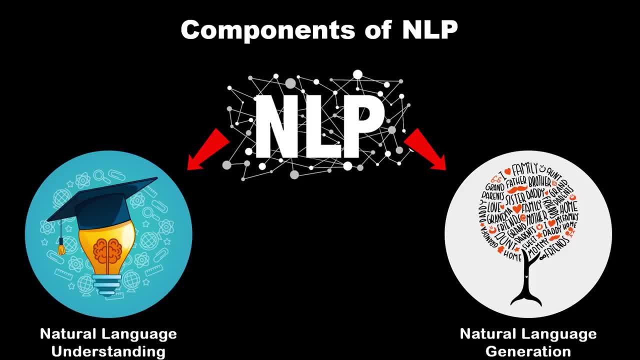 meaningful phrases and sentences in the form of natural language from some internal representation. Now, the natural language understanding is usually harder than the natural language generation, because it takes a lot of time and a lot of things to usually Understand a particular language, especially if you are not a human being. 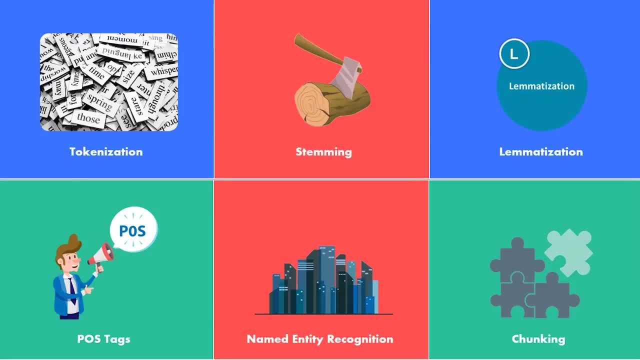 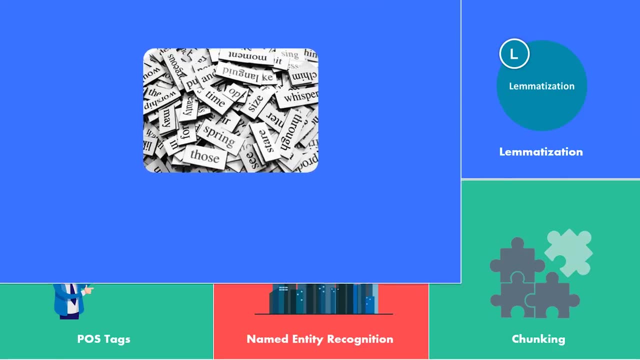 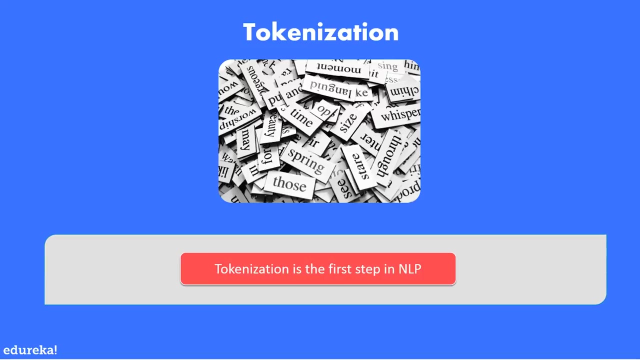 Now there are various steps involved in the natural language processing, which are tokenization, stemming, lemmatization, the POS tags, name entity recognition and chunking. Now, starting with tokenization: tokenization is the process of breaking strings into tokens, which in turn are small structures or units that can be used for tokenization. 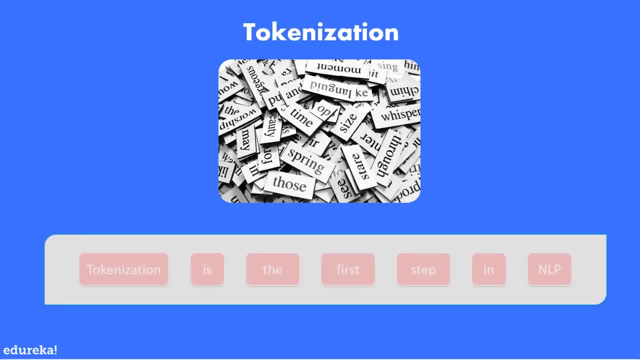 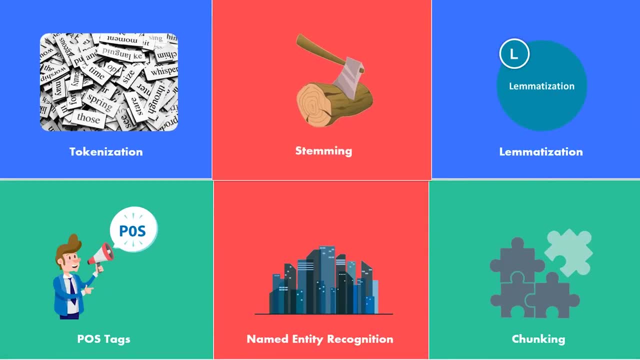 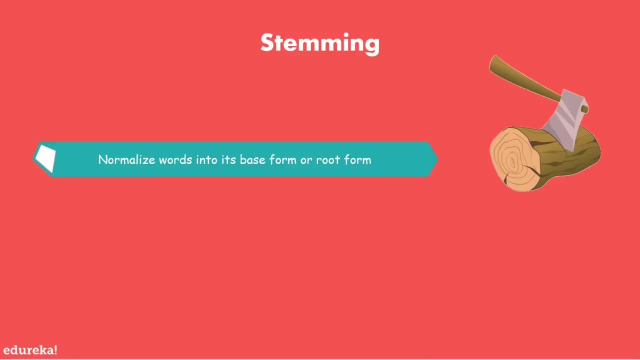 So if we have a look at the example here, taking this sentence into consideration, it can be divided into seven tokens. Now, this is very useful in the natural language processing part. Now coming to the second process in natural language processing is stemming. Now, stemming usually refers to normalizing the words into its base or the root form. 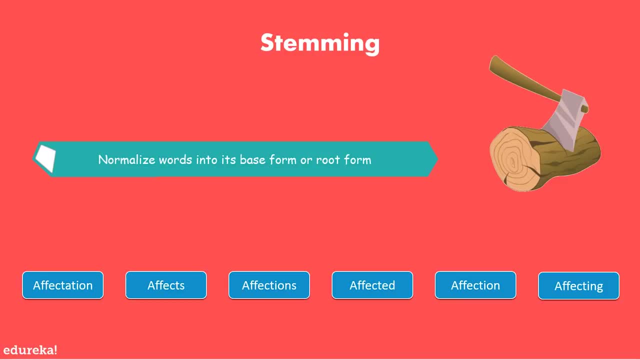 So if we have a look at the words here, we have affectation, affects, affections, affected, affection and affecting. Now, all of these words originate from a single root word and, as you might have guessed, it is affect. Now, stemming algorithm works by cutting off. 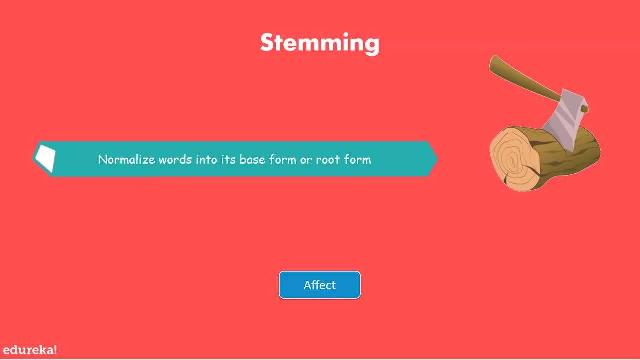 The end or the beginning of the word, taking into account a list of common prefixes, suffixes that can be found in an infected word. This indiscriminate cutting can be successful in some occasions, but not always. So let's understand the concept of lemmatization now. 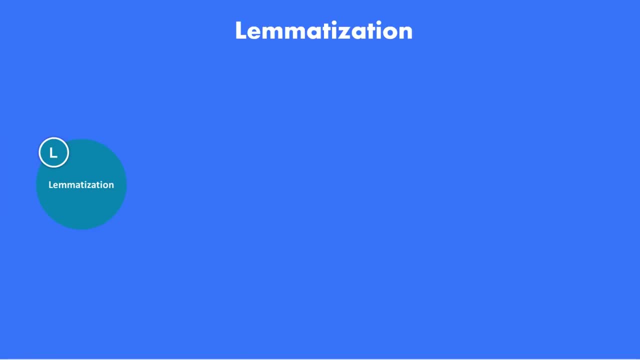 Lemmatization, on the other hand, takes into consideration the morphological analysis of the word. To do so, it is necessary to have a detailed dictionary which the algorithm can look through to link the form back to its originality. So, for example, let's say we have a word called lemma, which is an infected word, or the root. 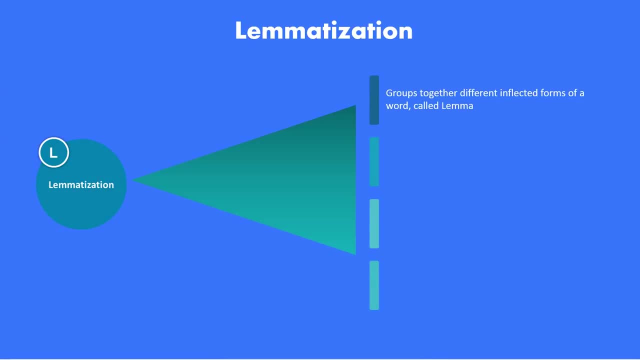 word, which is also known as lemma. Now, what lemmatization does is groups together different infected forms of the word called lemma and is somehow similar to stemming, as it maps several words into one common root. But the major difference between stemming and lemmatization is that the output of the 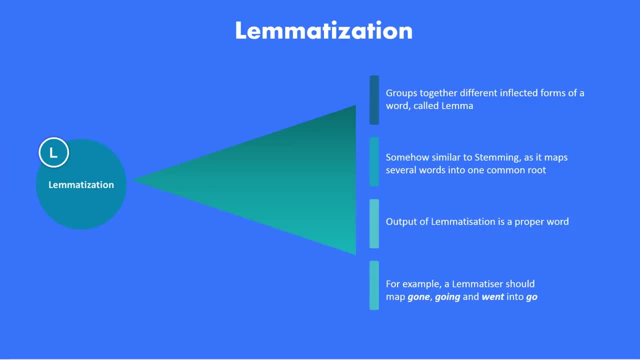 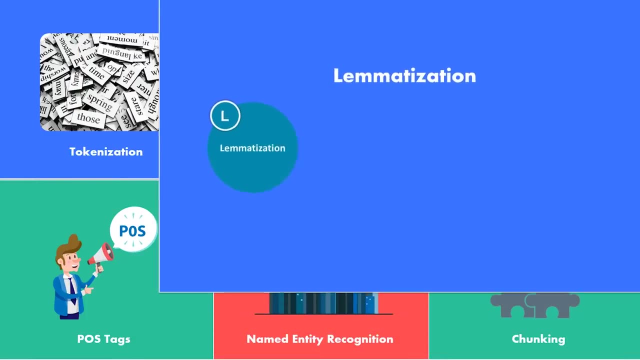 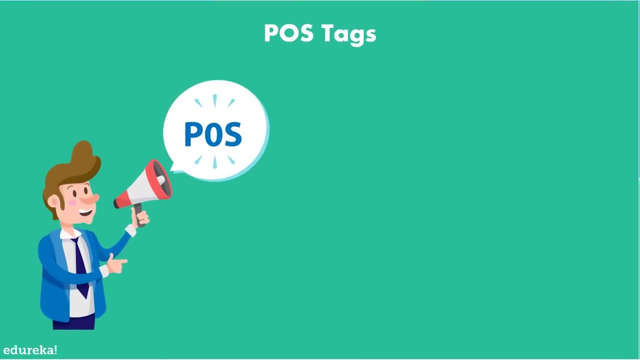 lemmatization is a proper word. For example, a lemmatizer should map the word gone, going and went into go. That will not be the output for stemming. Now, once we have the tokens And once we have divided the tokens into its root form, next comes the POS tags. 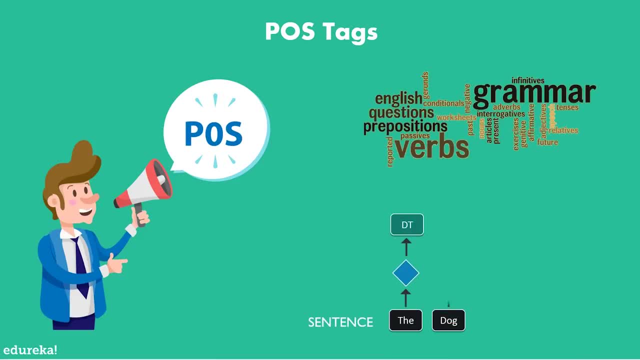 Now, generally speaking, the grammatical type of the word is referred to as POS tags or the parts of speech, be it the verb, noun, adjective, adverb, article and many more. It indicates how a word functions in meaning as well as grammatically within the sentence. 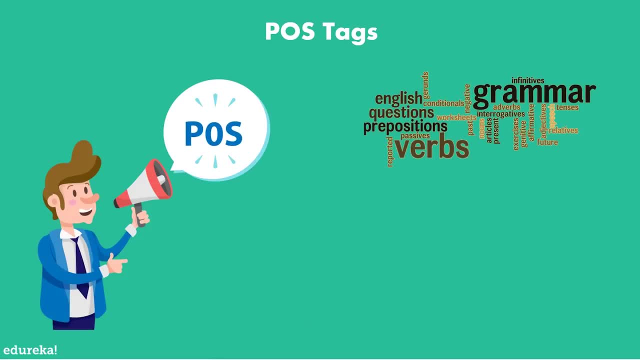 A word can have more than one part of speech based on the context in which it is used. For example, let's take the sentence Google something on the internet. Here, Google is used as a verb, although it's a proper noun. 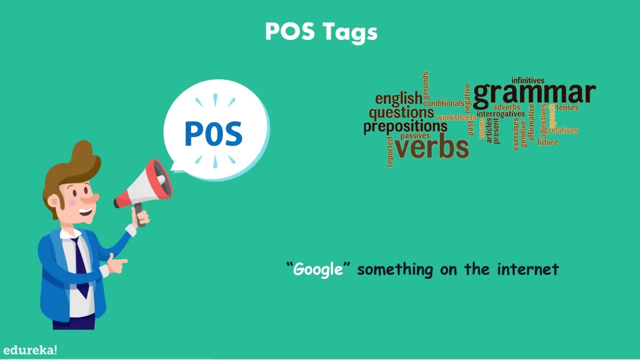 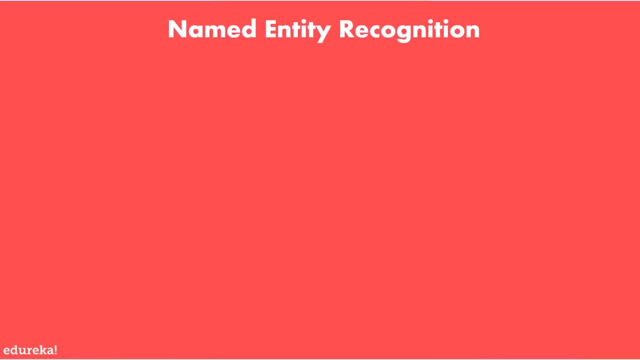 Now, these are some of the limitations, or I should say the problems that occur while processing the natural language. Now, to overcome all of these challenges, we have the name entity recognition, also known as NER. So it is the process of detecting the name entities, such as the person name, the company. 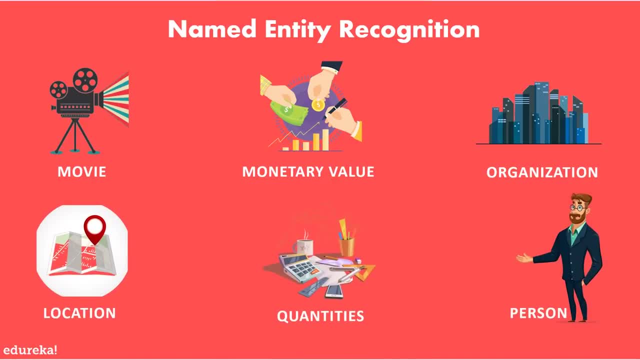 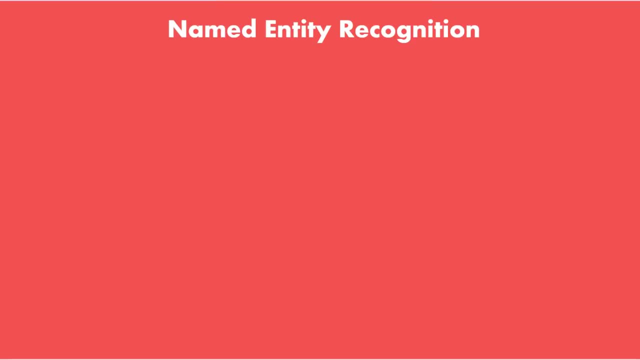 names, We have the quantities or the location. Now it has three steps, which are the noun phrase identification, the phrase classification and the entity disambiguation. So if you look at this particular example here, Google CEO Sundar Pichai introduced the 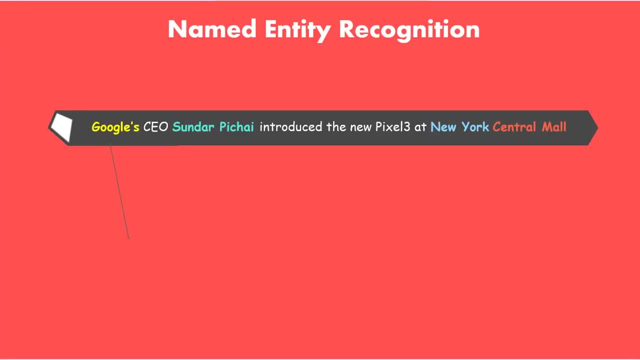 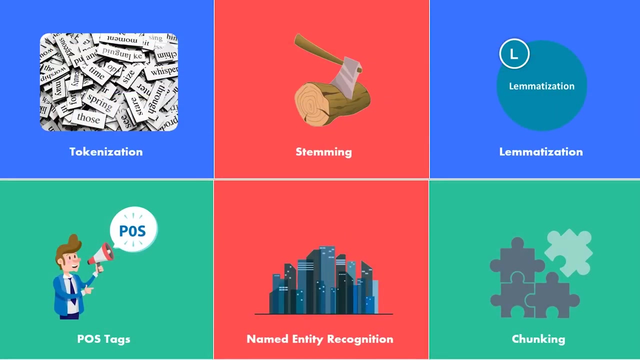 new Pixel 3 at New York Central Mall. So, as you can see here, Google is identified as a organization, Sundar Pichai as a person, We have New York as location and Central Mall is also defined as an organization. Now, once we have divided the sentences into tokens, done the stemming, the limitization, 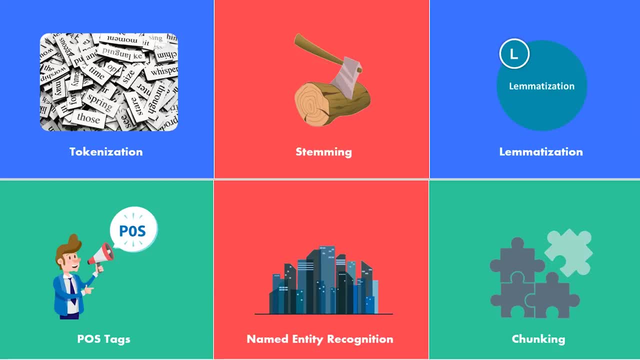 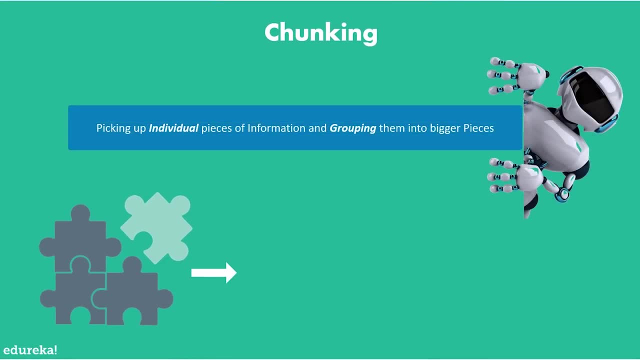 added the tags, added the name, entity recognition. It's time for us to group it down. Let's go back together and make sense out of it. So for that we have chunking. So chunking basically means picking up individual pieces of information and grouping them together. 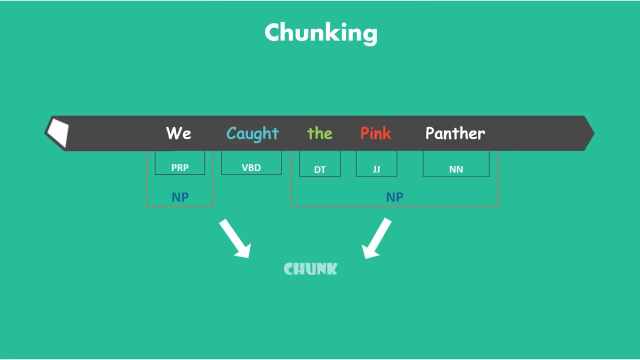 into the bigger pieces. Now, these bigger pieces are also known as chunks. In the context of NLP, chunking means grouping of words or tokens into chunks. So, as you can see, here we have pink as an adjective, panther as a noun and D as a denominator.